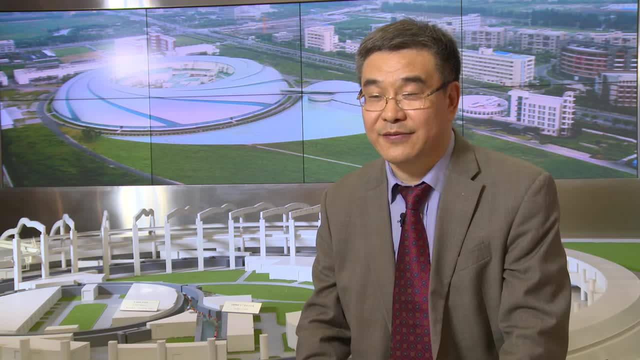 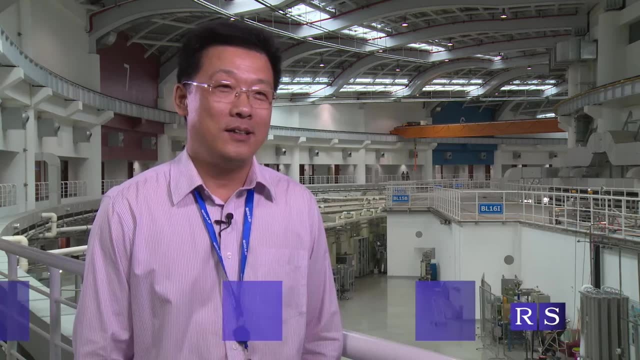 movement lighting. It's providing high brightness and high flux to the scientists to do research. so worldwide it is world-class facility. Zao� long�� di产 ŏu port perché. Shanghai Synchrotron Radiation Facility is one of the most advanced medium energy lights source in the world. It has highest energy in the medium energy facilities. It provides the high brightness and high flux to the scientists to do research World-wide. it's a important facility. 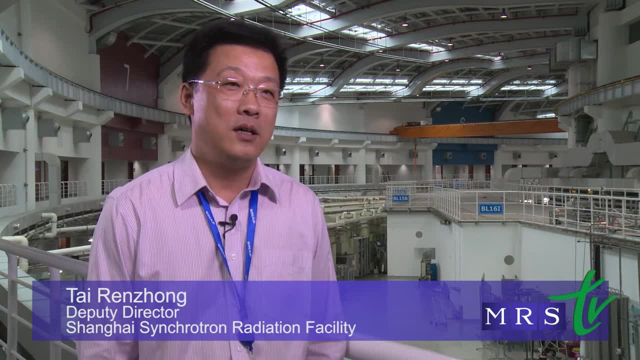 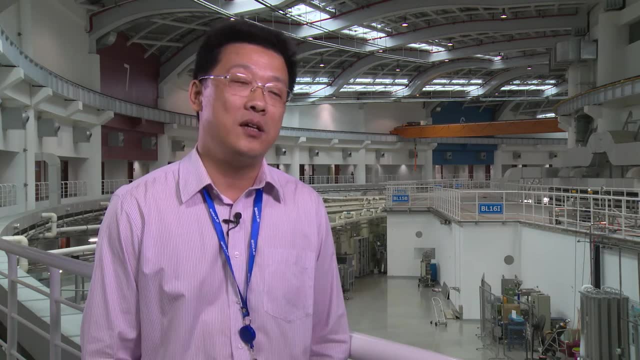 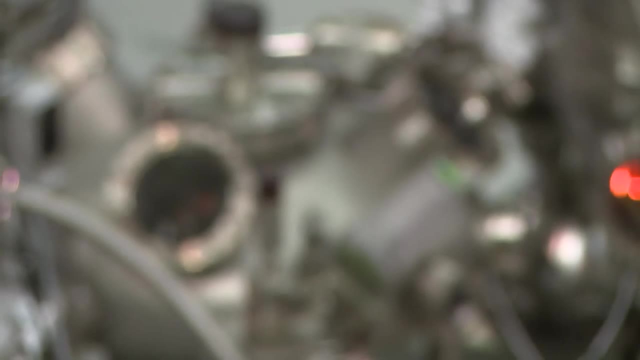 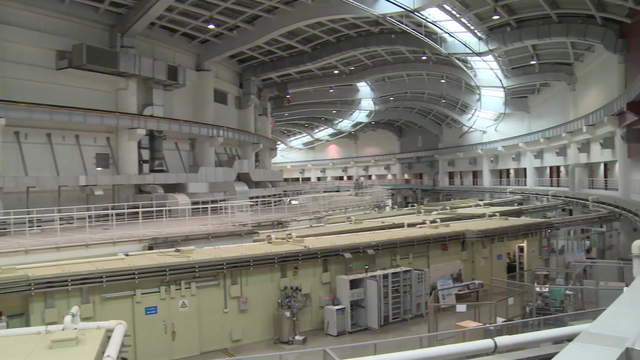 radiation facility in its first phase constructed seven beam lines with excellent output so far. Just recently, six new additional beam lines have been opened to users. 16 more state-of-the-art beam lines will be built within coming five to six years in Shanghai Synchronization Facility. 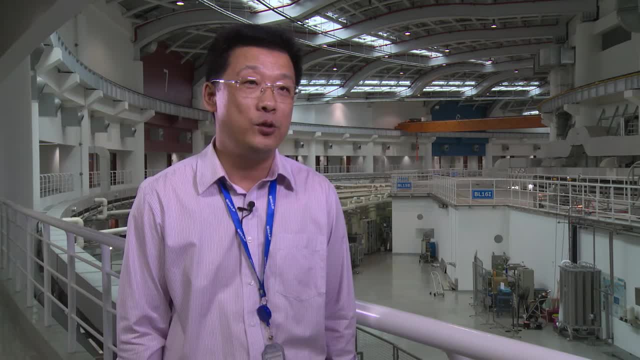 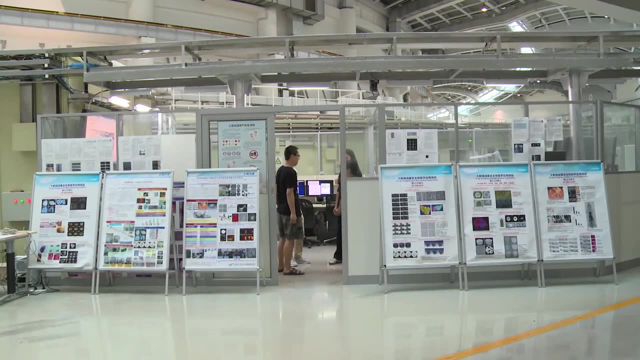 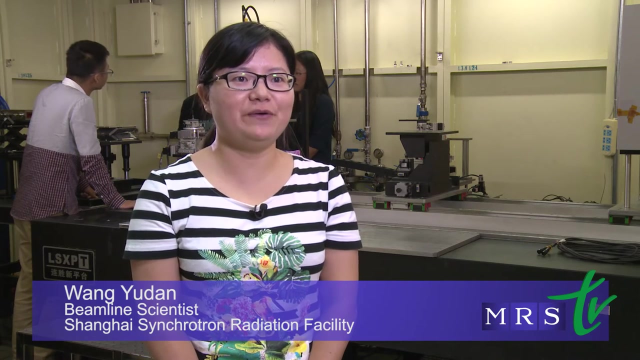 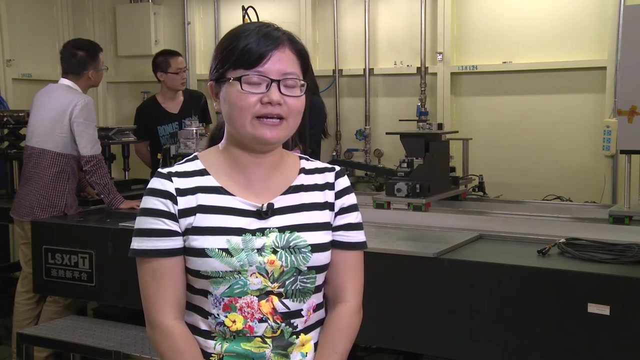 This is a so-called SSRF Phase II beam line project. A couple more contracted beam lines are also scheduled In BL13W. the X-ray imaging is a powerful tool for material science. One of the advantages is we can observe the sample in situ or in operandum during processing and operating. 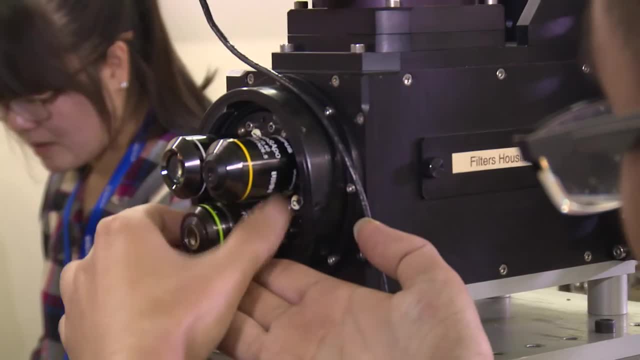 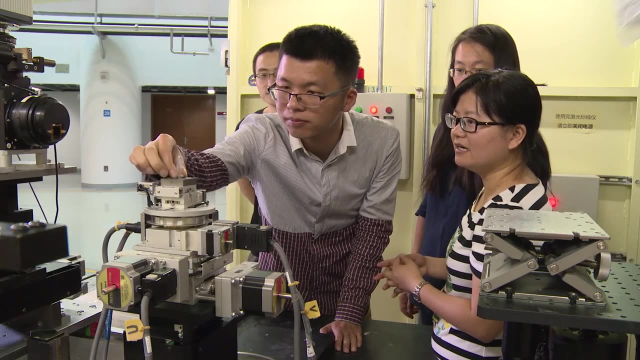 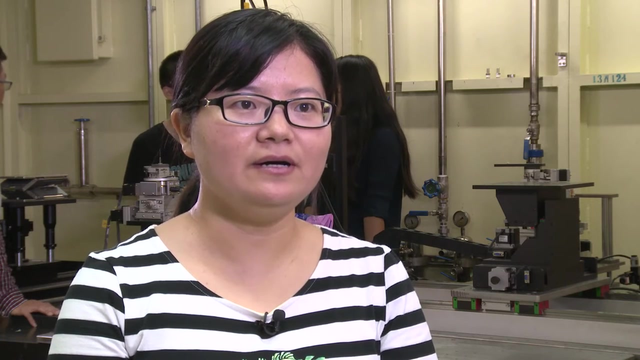 Another point is: using microtomography, we can observe the structure of the materials and then quantitatively measure the structures. Almost half of the beam time is assigned for material science in various areas, including alloy, polymer, biomaterials and so on, For example, during the solidification processing. 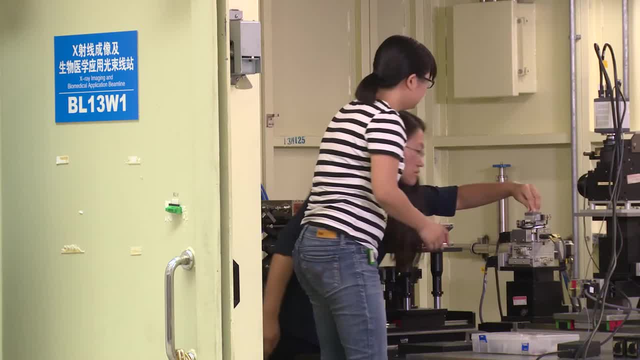 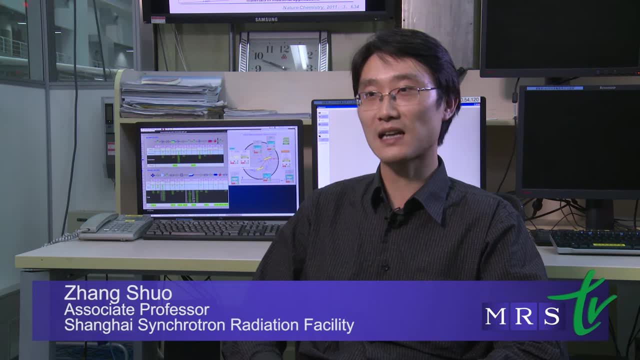 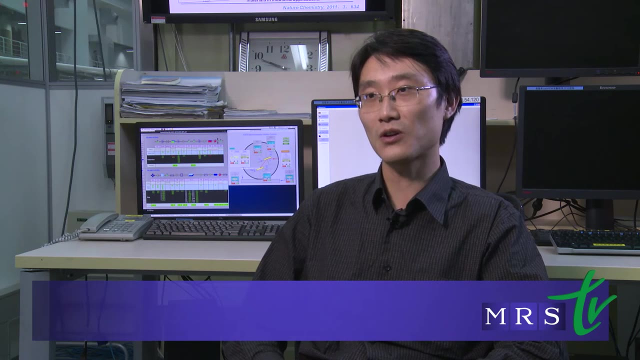 we can observe the dendrite growth in situ. This helps us better understand the mechanism of the dendrite growth. The BL13W was designed for X-ray absorption phase structure technique. It uses regular light source. The maximum photo flux can be 10 to the power of 13 per second. 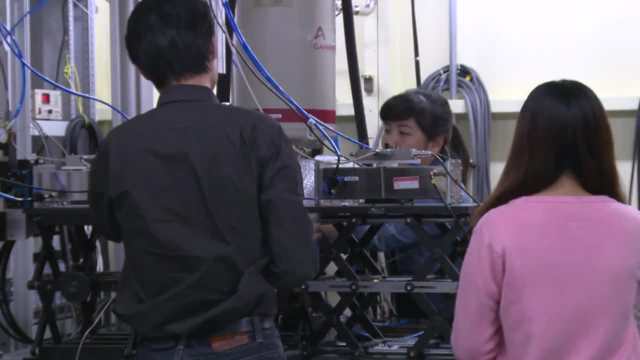 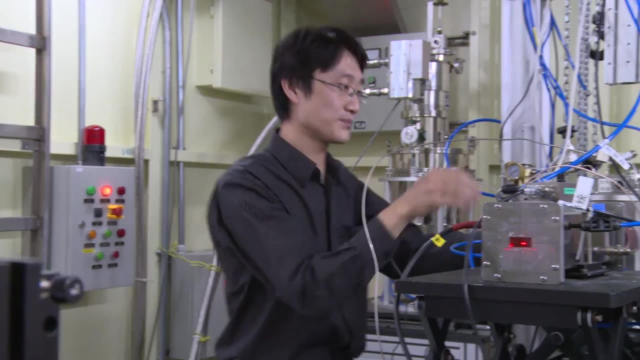 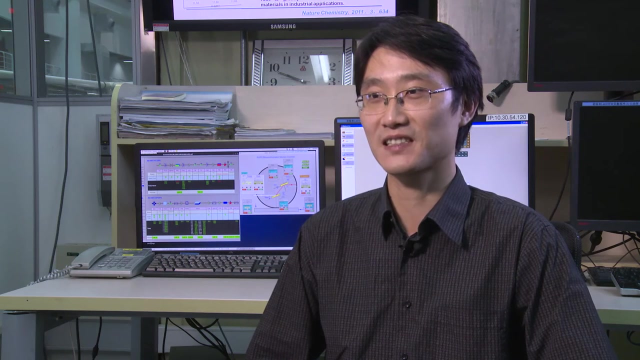 The energy range of this beam line is from 4,000 EW to 15,000 EW, covering the most of elements. The SAFSS technique has wide applications in the fields of physics, chemistry, country biology. environmental science, especially, is very important for catalysts. 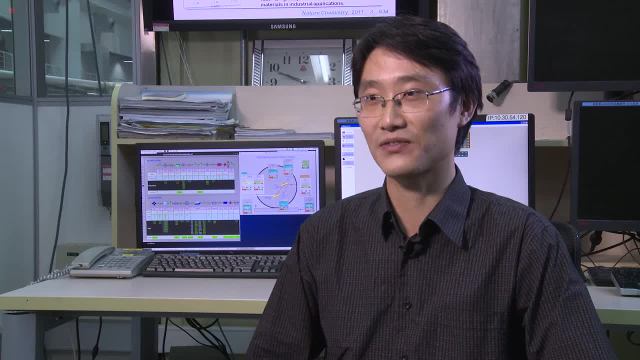 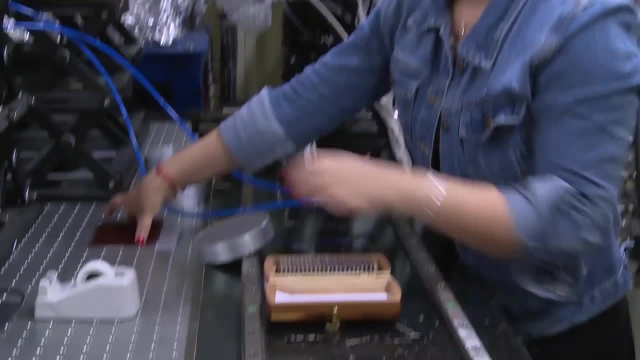 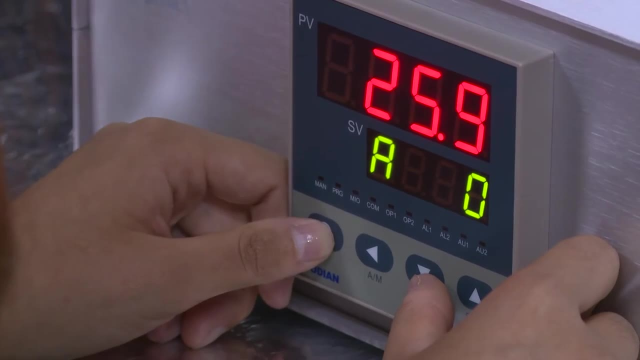 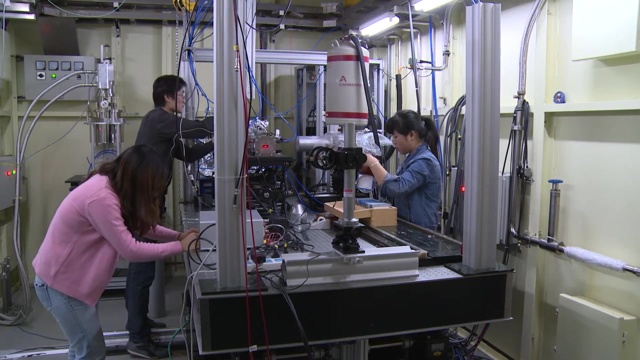 Many Chinese users gave excellent research in this field. The users came here and they usually perform these experiments under the high temperature and also in the presence of reaction gas. By these experiments the users can understand what kind of microstructure and what kind of electronic structure are suitable for chemical reaction. 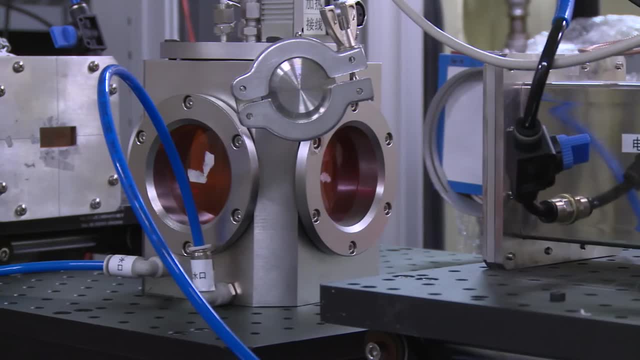 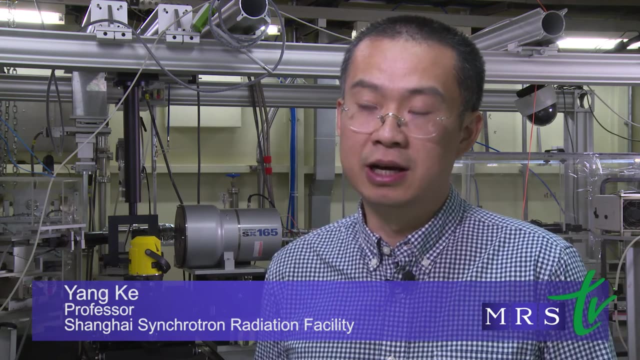 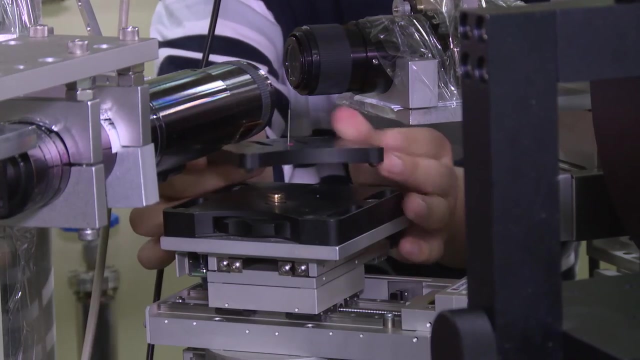 It's very useful to design high-efficient and low-cost catalysts. Microfocus beamline can provide a very small beam size, just several microns beam. That's very important for the material research because sometimes the sample is quite small or the sample area is quite small. 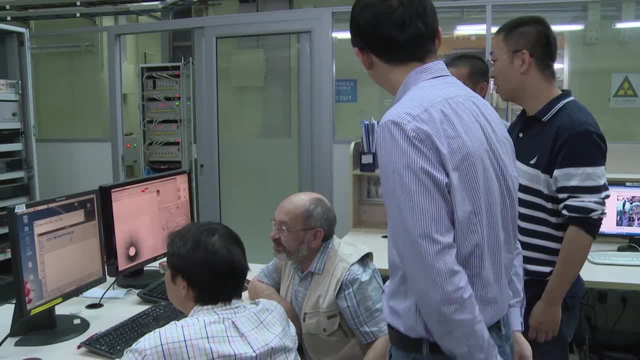 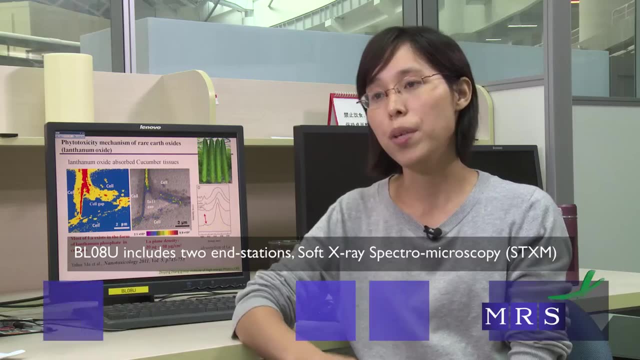 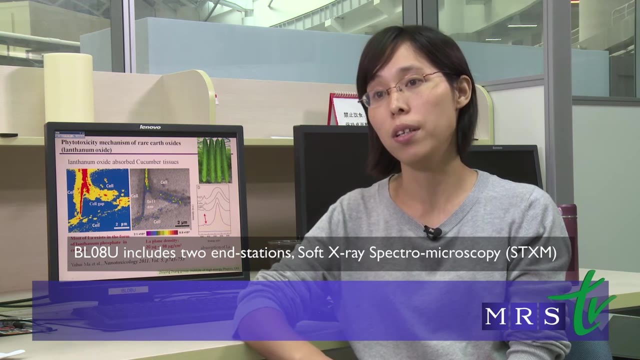 For example, though, For the silk, the fiber and some pores in the sample. So we need a very small beam to study the materials. In BL08U there are two interstations. One is soft X-ray spectral microscopy. 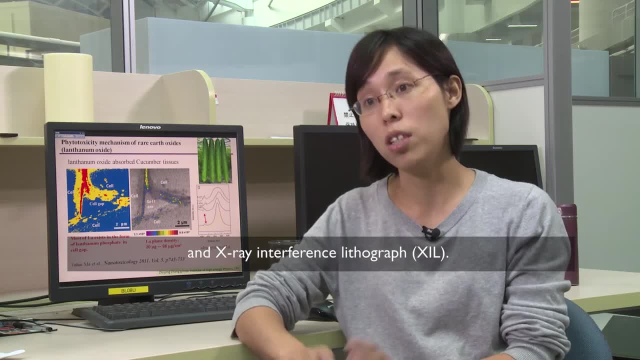 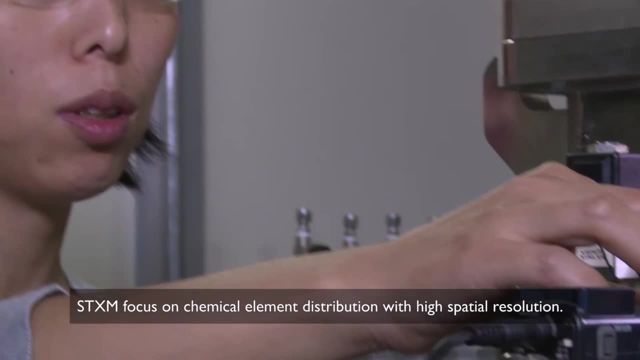 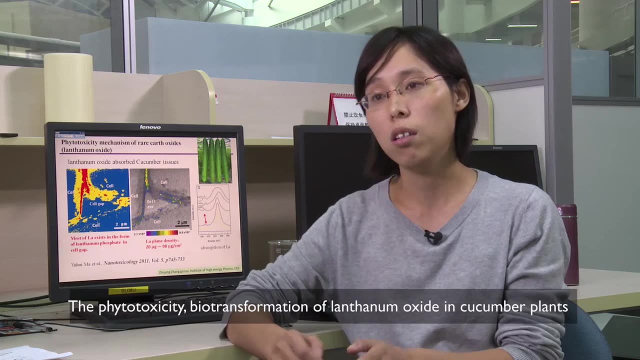 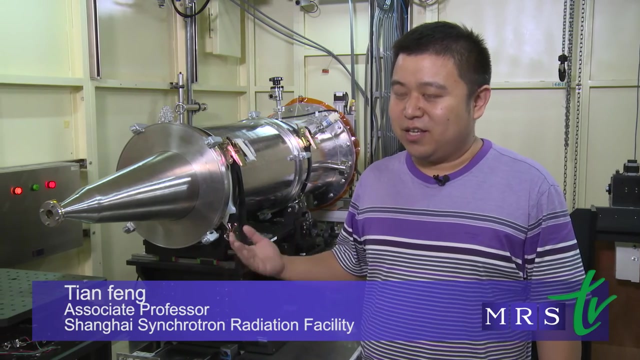 and the other is X-ray inverse lithography. X-ray spectral microscopy functions at quantitative maps of chemical element distributions with high spatial resolution. The phytotoxicity mechanisms of lithium oxide nanoparticles have been studied by this technique. This is BL16B1 station and the whole name of this station. 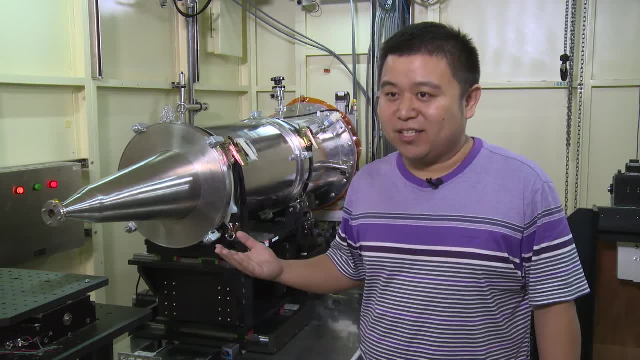 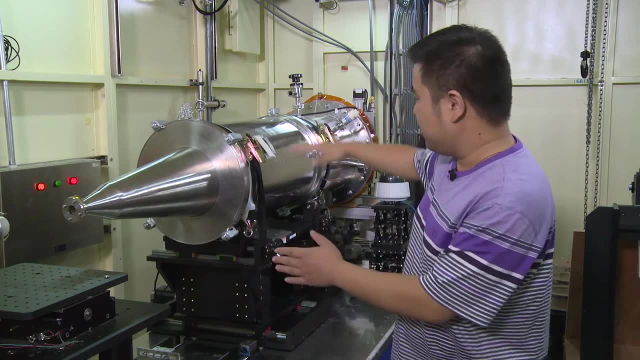 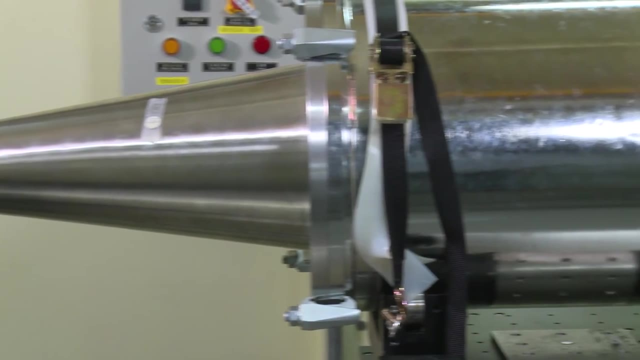 is small angle X-ray scattering beam line. When we do experiment, we put a sample here and scattering occurs. After a vacuum tube. the scattering information will be. It will be tested by the detector. We can get the inner structure of the polymer. 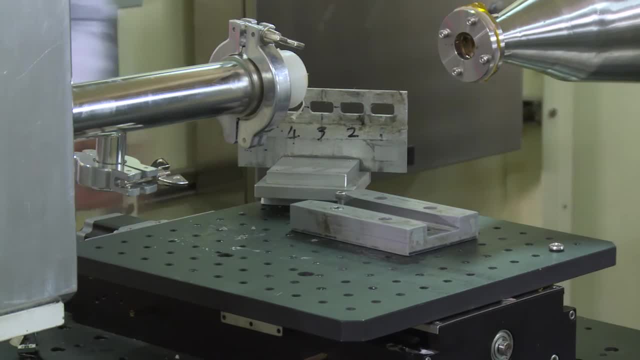 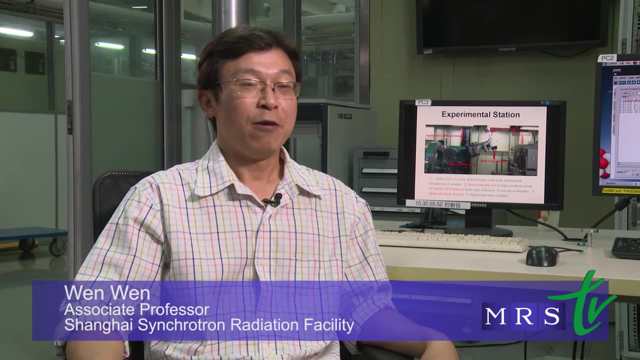 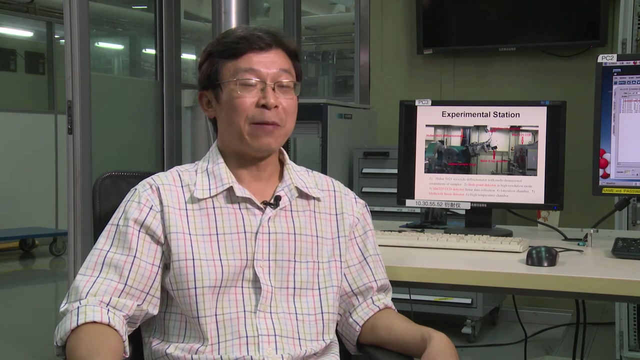 by analysis the scattering information. BL14B1, which is a general purpose X-ray diffraction beam line. it's mainly equipped with a Huber 5021 diffractometer, allow multidimensional orientation of samples. It has equipped with three detectors.